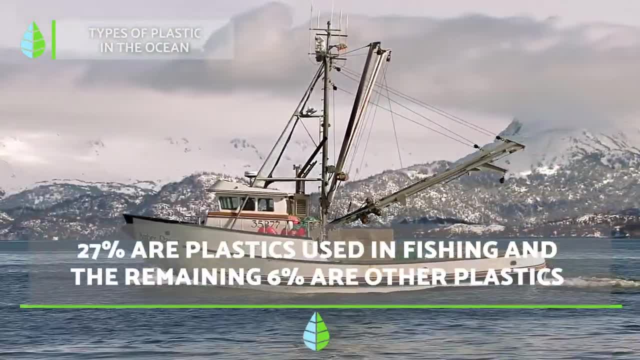 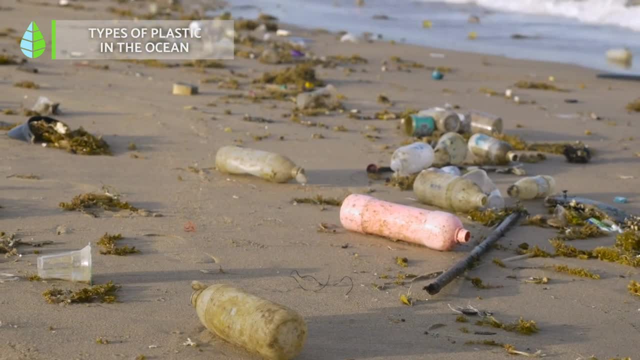 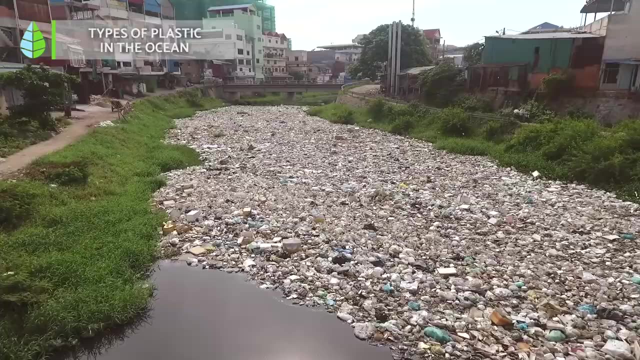 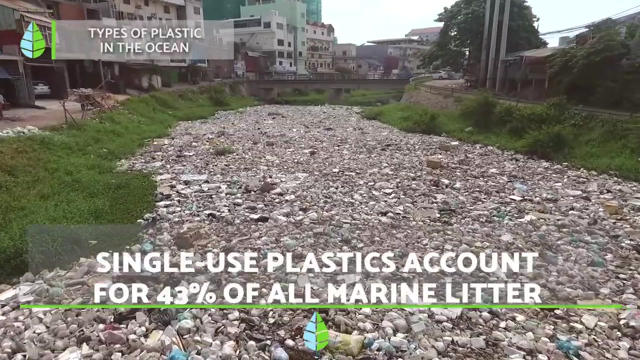 plastics that have been found on the beaches and seabed are lids, bottles, cigarette butts, cotton butts, snack wrappers, hygiene items, plastic bags, tupperware, straws, plates, glasses, balloons and food containers. These products represent 86% of single-use plastics. 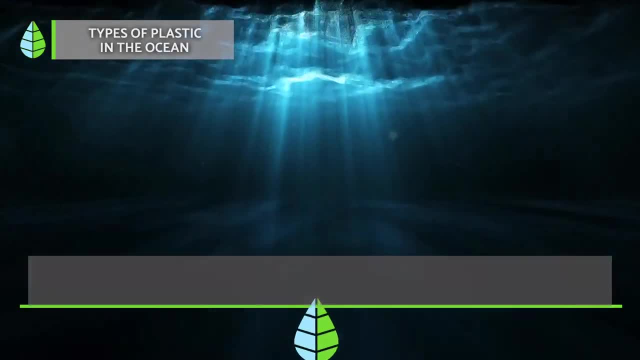 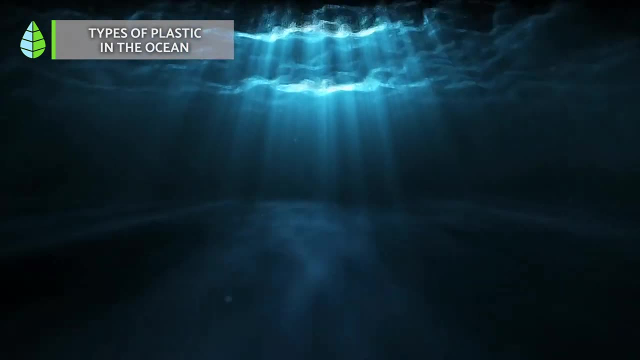 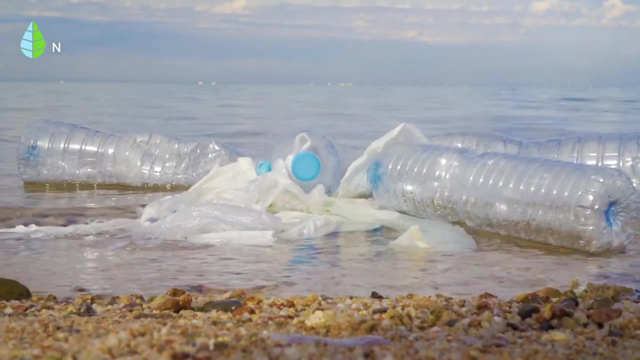 or 43% of all marine litter. Some have even been found 10,000 meters in depth. However, some areas, which are called plastic islands, have been identified where they have a great concentration of plastic. Before we continue, let's put you to the test. How much plastic is already accumulated in our 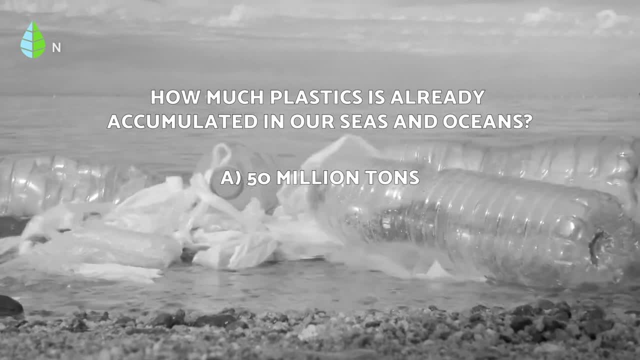 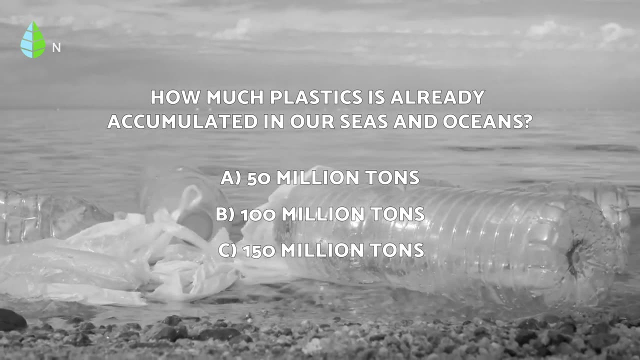 oceans. Is it A- 50 million tons, B- 100 million tons or C- 150 million tons? Think about it, because I'm sure you've all heard the word plastic. I'm sure you've all heard the word plastic. 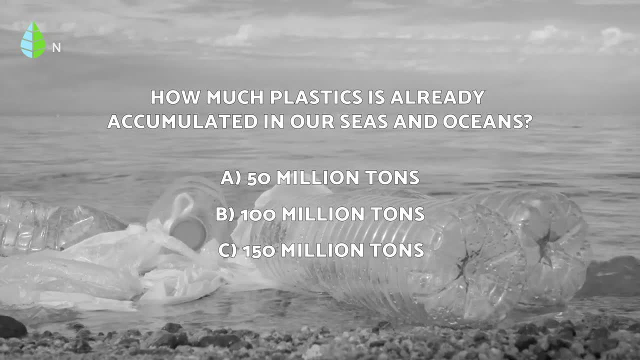 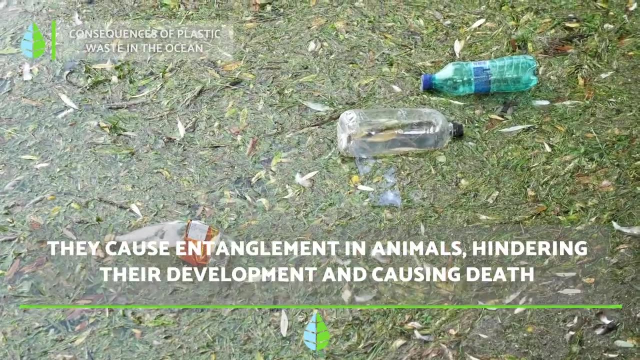 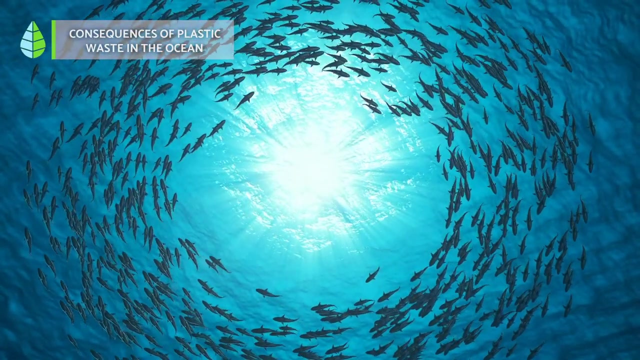 At the end of the video, you'll be able to find out if you were right. Consequences of Plastic in the Ocean. On one hand, plastic waste causes entanglement in certain marine animals, hindering their development and even causing their death. Some of these animals mistake the pieces of plastic for. 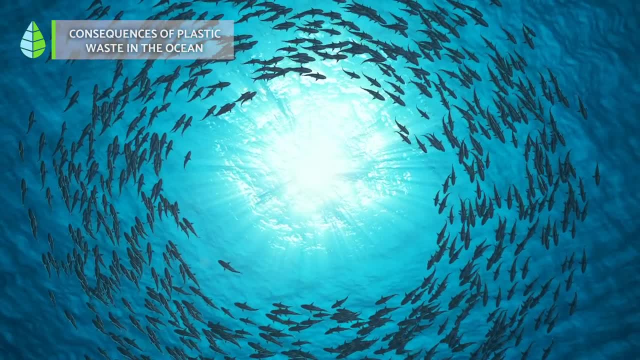 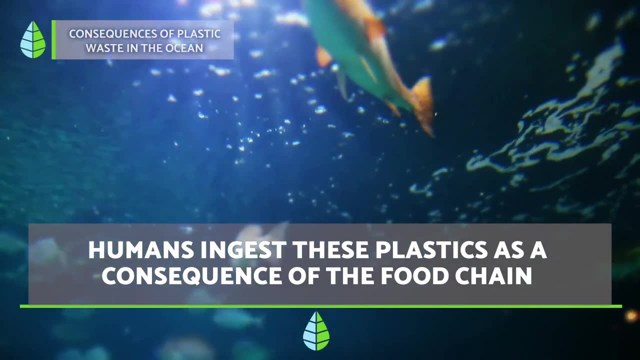 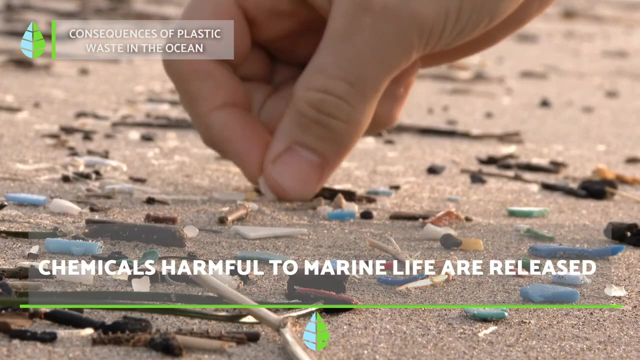 their usual food, something that can block their stomach and also lead to their death. Likewise, human beings also ingest these materials as a consequence of the food chain. In addition, in the long process of decomposition, microplastics and nanoplastics release chemicals that are harmful. 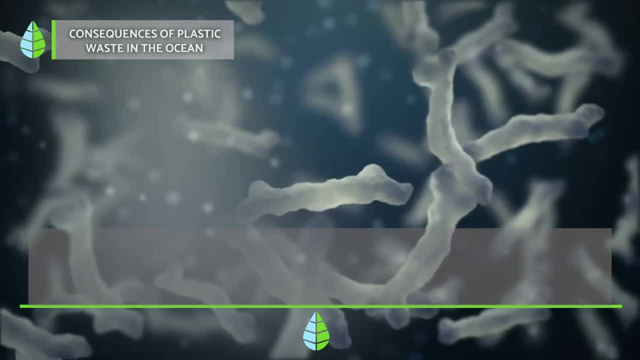 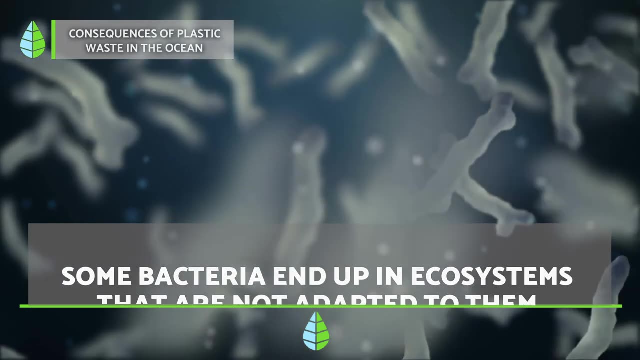 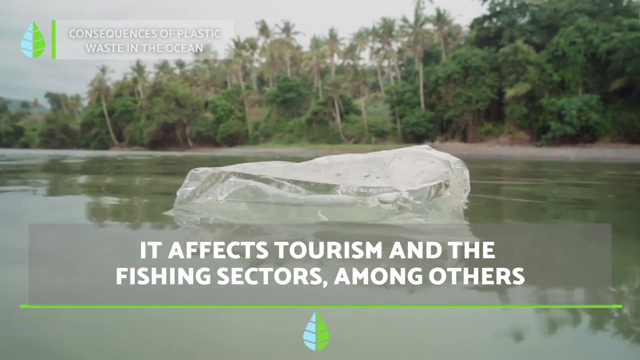 to life in ocean waters. On the other hand, there are some species of bacteria that develop on plastic which moves freely and take them to ecosystems that they're not adapted to. And, lastly, plastic waste in the ocean also has a negative impact on our economy. 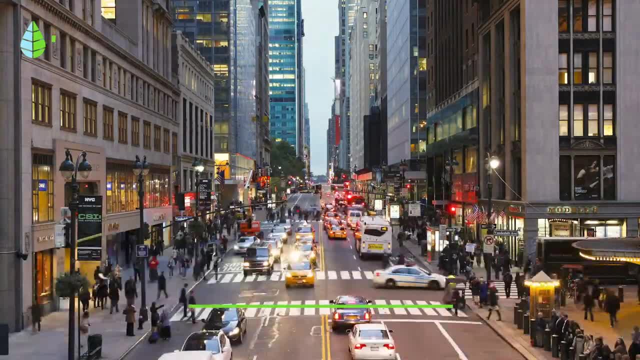 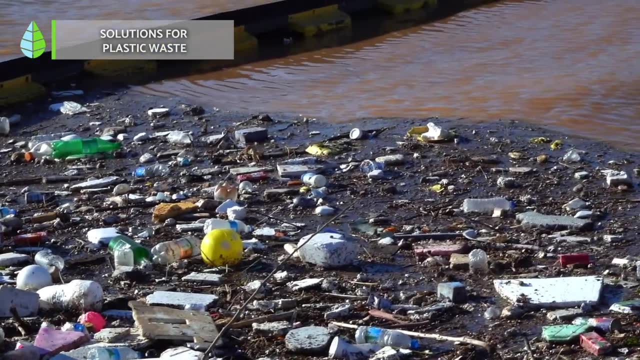 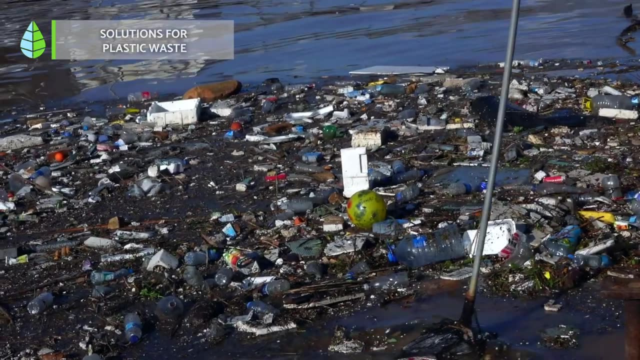 especially the tourism and the fishing sectors. Solutions for Plastic Waste in the Ocean. The solutions must involve producers, consumers and those who manage waste, but of course, it has to be supported by the governments. The main solutions we propose are Reduce the consumption of plastic and avoid using single-use plastic. In fact,